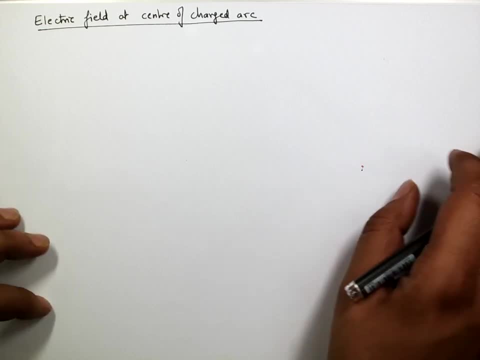 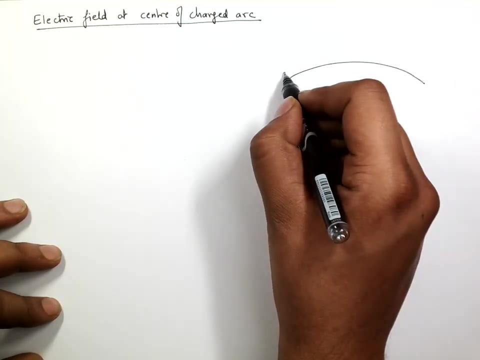 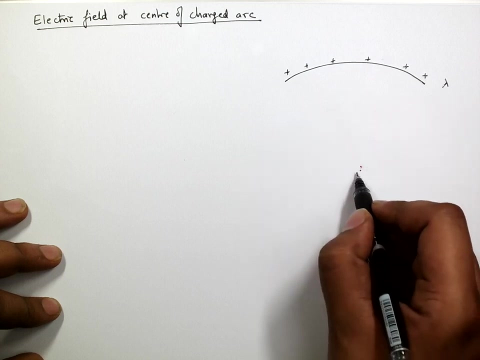 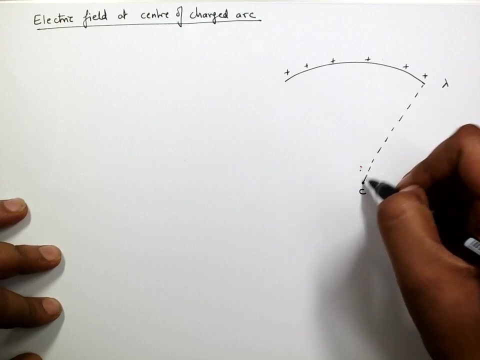 Electric field at center of a charged arc. Suppose we have a charged arc, a uniformly charged arc, Let's say charge density lambda, and we need to find electric field at its center, which is the center of the circle from which this arc is taken. Now what I do. first, 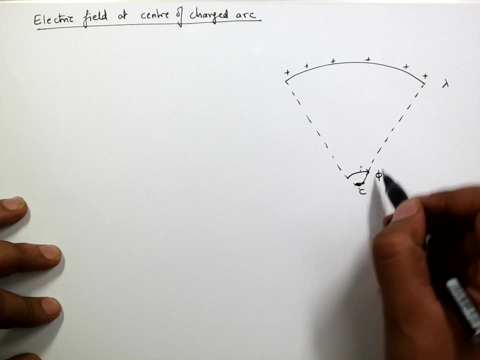 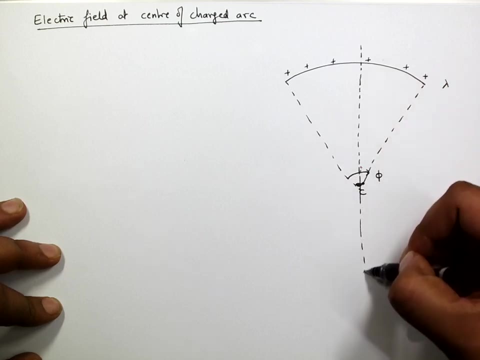 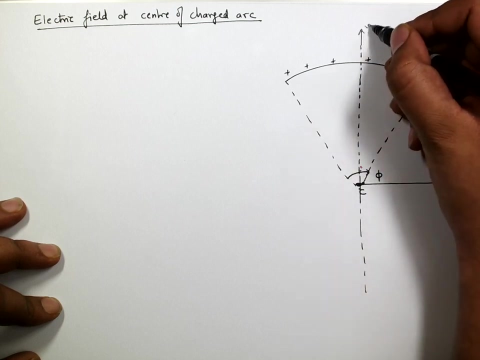 is. let us suppose that this angle is phi. Let us take the angle bisector of this arc and let us suppose perpendicular to this angle bisector is x axis and this axis is y. Now, by symmetry considerations we can see that the net electric field must be along the angle. 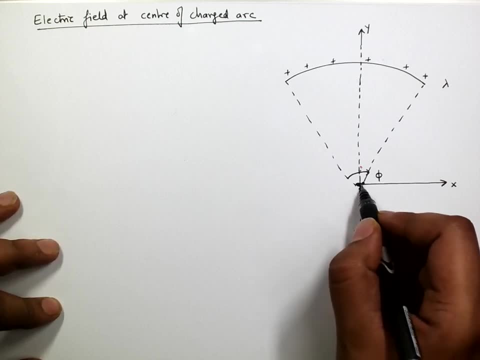 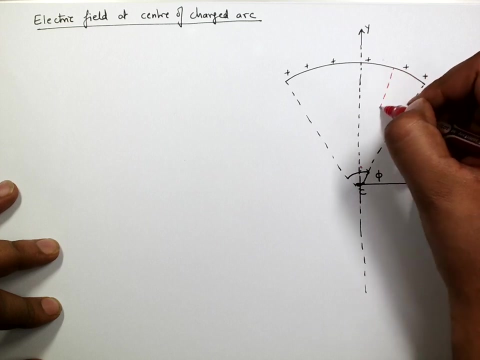 bisector direction. So net electric field must be along angle bisector direction. because of this, The symmetry considerations, because the electric field components along x direction, will cancel out. Now let us take a charge element. Let us take a charge element at an angle theta. 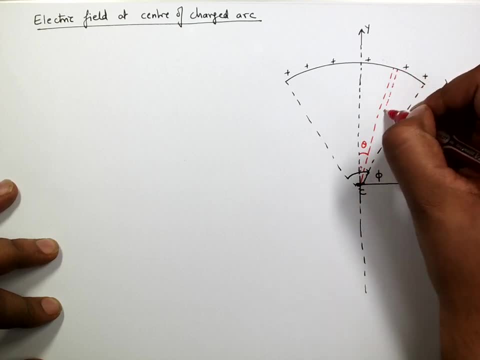 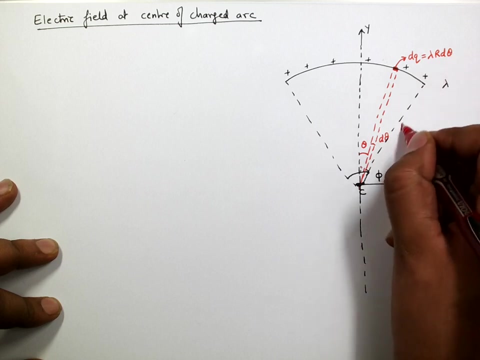 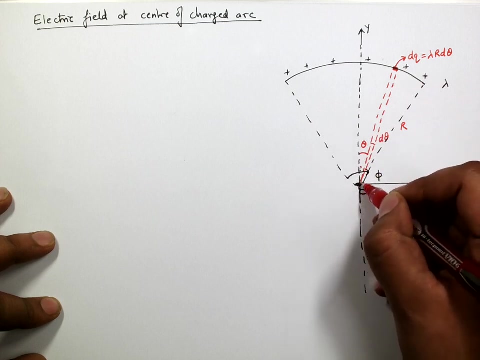 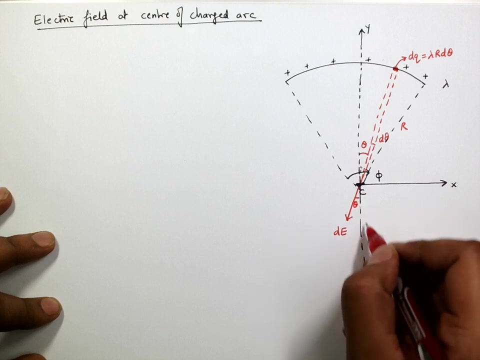 of so sending an angle of d theta at the center. So the charge on this element, dq, will be lambda r d theta Here. r is the radius of this arc. Now electric field at center because of this charge element will be, let us say, d e and this angle will be theta. Now d e will have two components. 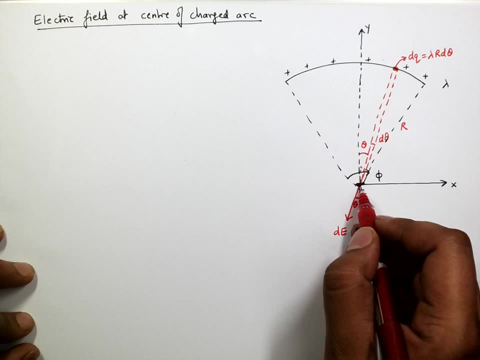 d e cos theta and d e sin theta, and ideally we need to integrate both of them. but however, d e sin theta, which will be the component along x direction, will be lambda r d theta. Now, if we integrate over this arc by symmetry, they will cancel out. 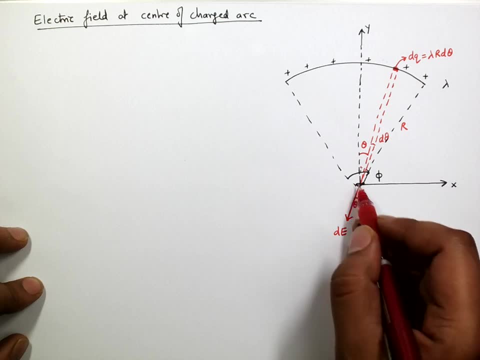 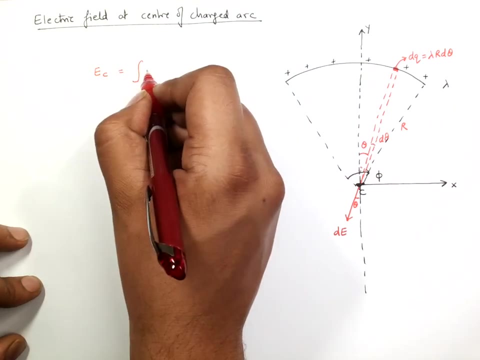 So we just need to calculate, integrate the d e cos theta and find electric field at center. So electric field, the delta along x direction will be integration of d e cos theta, And this we can do. as now, d e will be a divided by r d theta, So here r d theta is the hot. 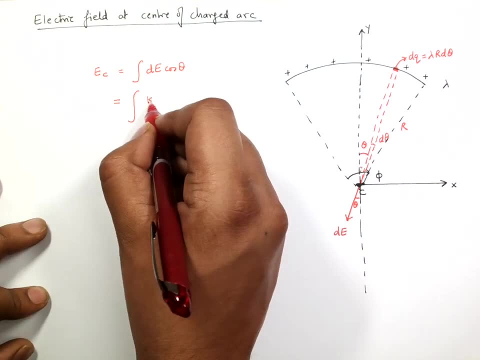 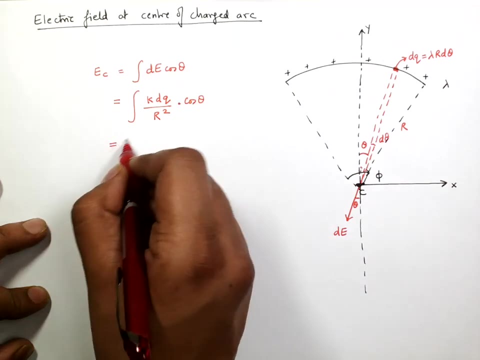 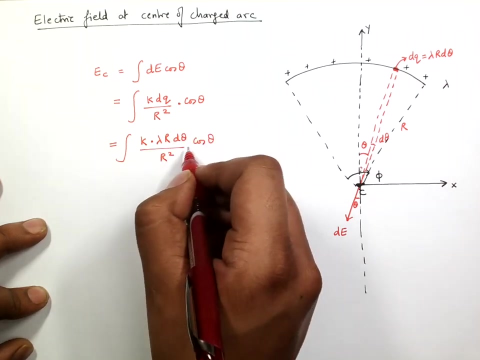 electric field at center. So electric field at center will be integration of d e cos theta And t BB will be right acting r square multiplied by cos theta. so this is integration of k lambda r d theta divided by r square. integration of cos theta r cancels out. so this is k lambda by r integration of. 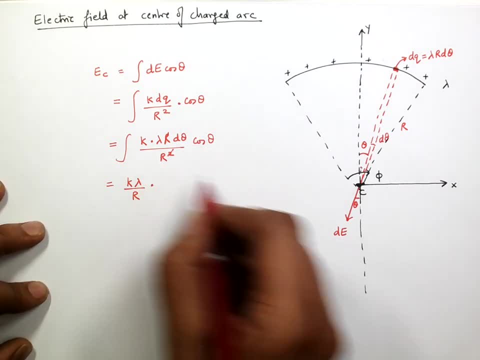 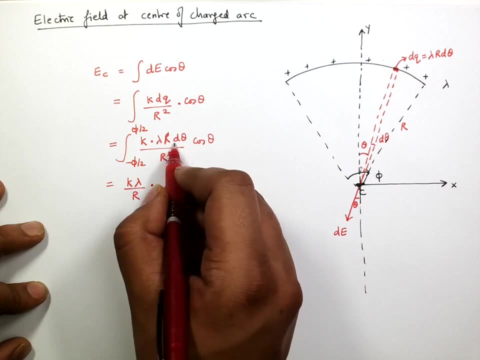 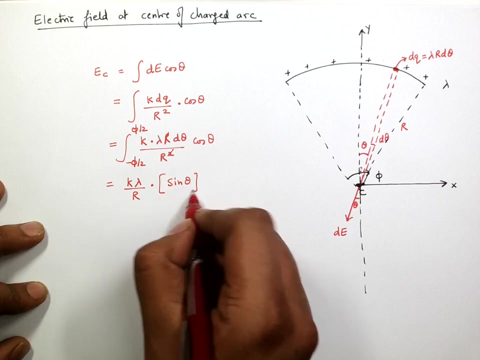 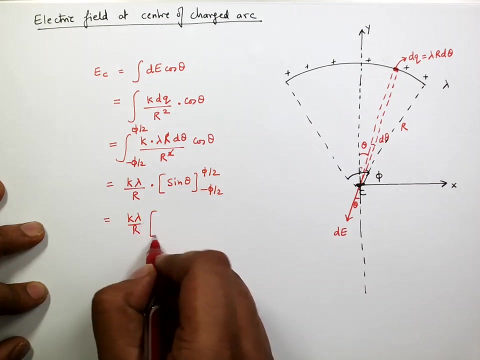 cos theta d theta, which is sin theta. now limits for angle theta are minus 5 by 2 to 5 by 2, so this is integration of cos theta d theta, which gives us sin theta, and we have limits minus 5 by 2 to 5 by 2, so this gives us k lambda by r sin of 5 by 2, minus sin of minus. 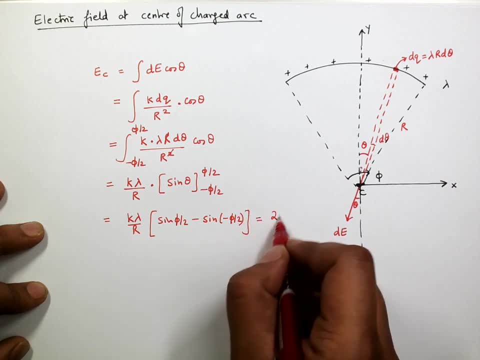 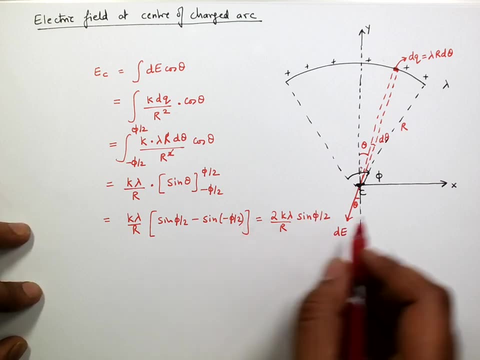 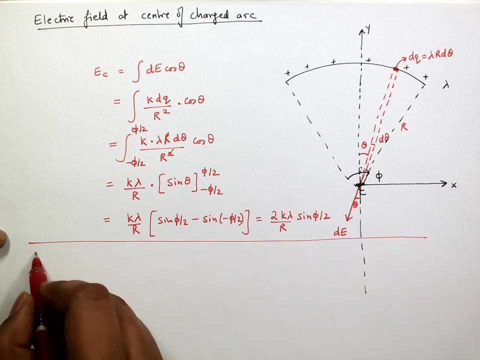 5 by 2, which is 2k lambda by r, sin of 5 by 2. so this is the electric field at the center of this charged arc. now some special cases. first, if we have a closed complete circle of radius r with charge density lambda, then 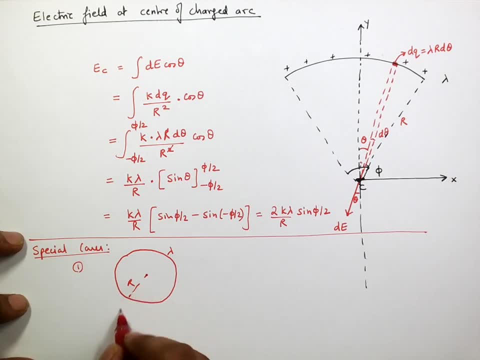 by symmetry considerations as well, we can say that it will be 0 and by this formula the electric field will be 2 pi, so sin of pi, which is 0, and it checks out. second, if we have a semicircular arc, we have a semicircular arc and we need electric field at center, then 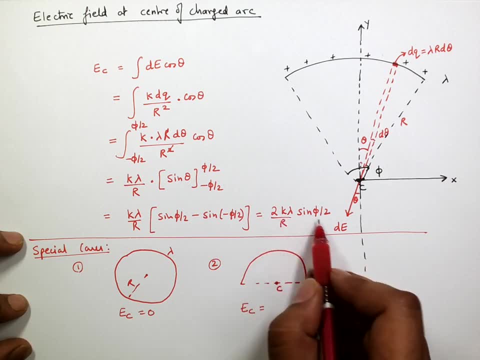 electric field will be 2k lambda by r, sin of now phi is equal to pi, so sin of pi by 2, which is 1, so this will be 2k lambda by r. third is finished. third is done. we have a quarter arc. we have a quarter arc and obviously, direct. 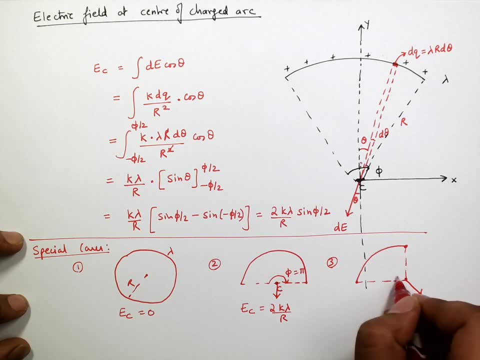 shine will be in this direction. if you have a quarterly käyt, than electric field will be in long the angle bisector, which is what we are doing- forty five degree, and this electric field will be to k lambda by r. in this case, phi is equal to 5 by 2, so sine of 5 by 4 sine.